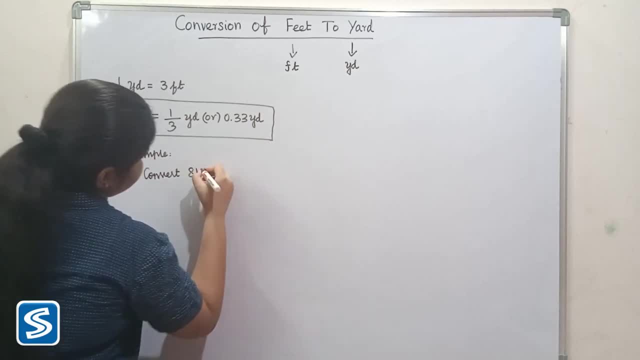 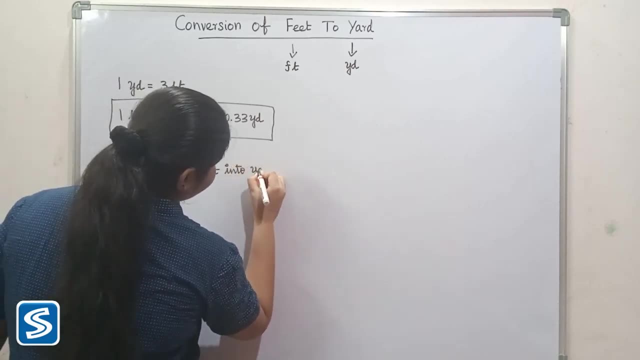 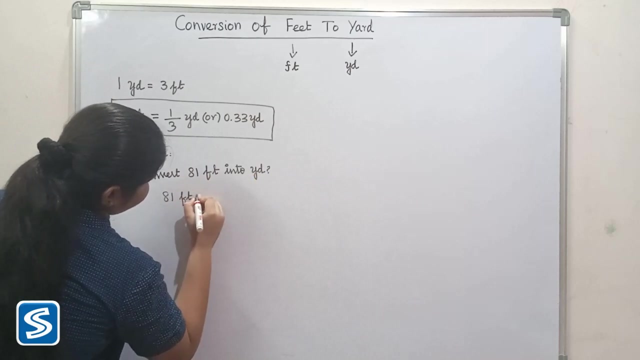 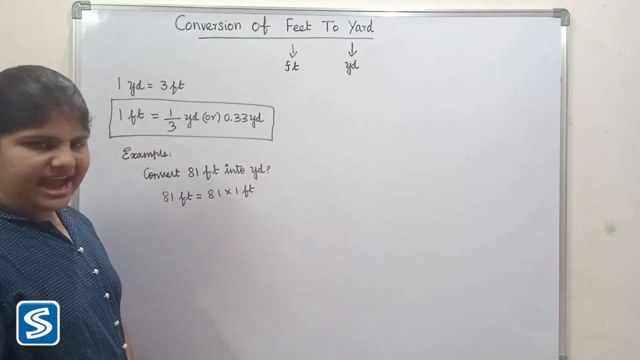 Now we have to substitute 1 by 3 yard in the place of 1 feet. 81 feet into yard. 81 feet can be written as 81 multiplied 1 feet. Now we have to substitute 1 by 3 yard in place of 1 feet. 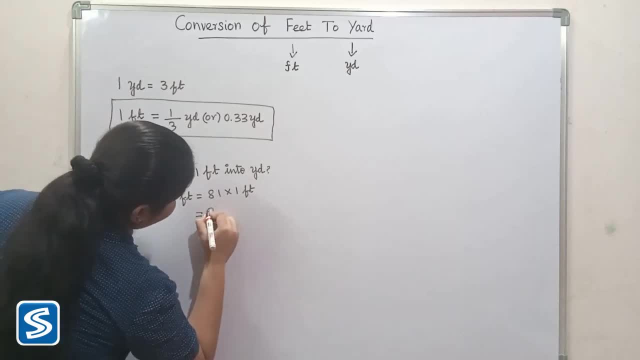 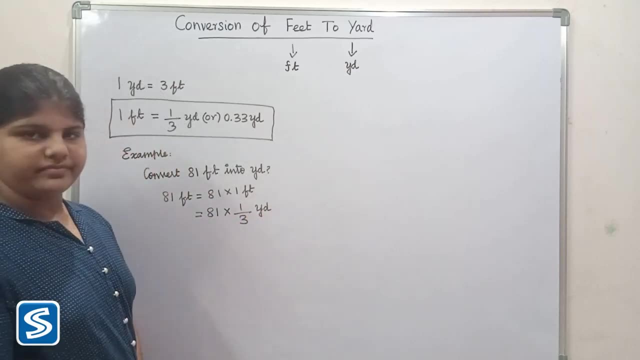 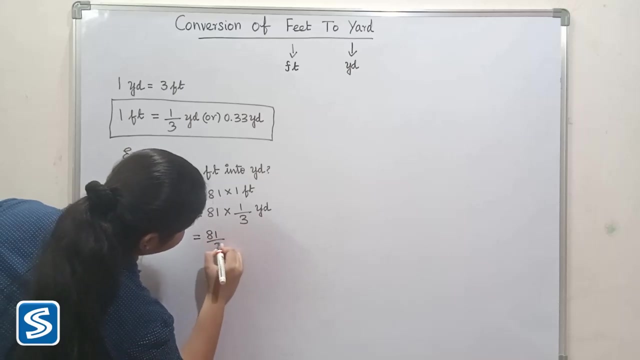 1 by 3 yard, 1 by 3 yard, 1 by 3 yard. So 81 multiply 1 by 3, yeah, 81 multiply 1 will be 81.. So 81 by 3, yeah. 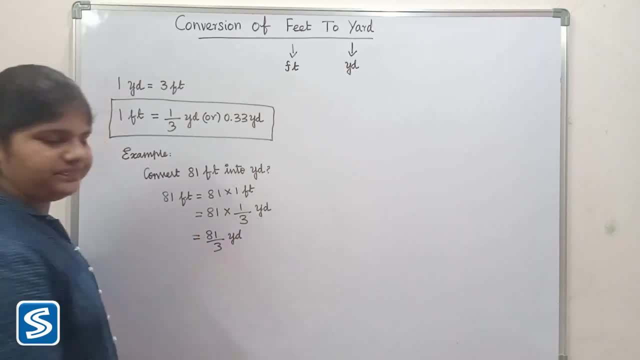 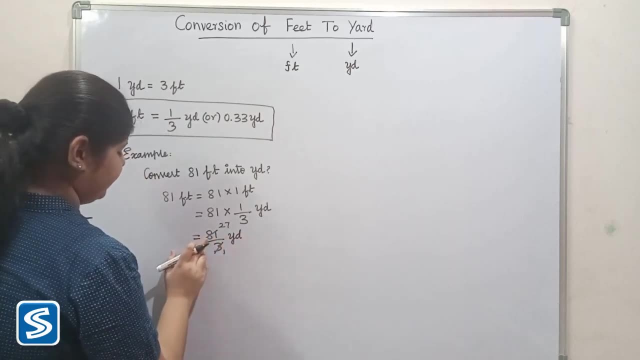 Now we have to divide 81 by 3, yeah. So 3 1's are 3,, 3 27's are 81. So when we divide 81 by 3, yeah, our answer will be 27,. yeah. 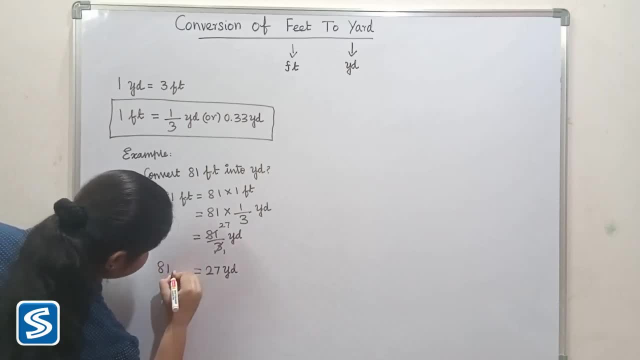 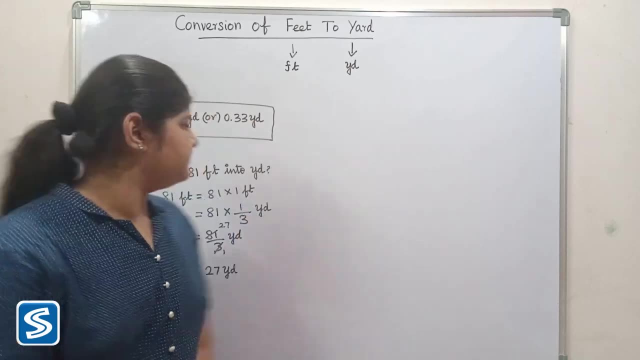 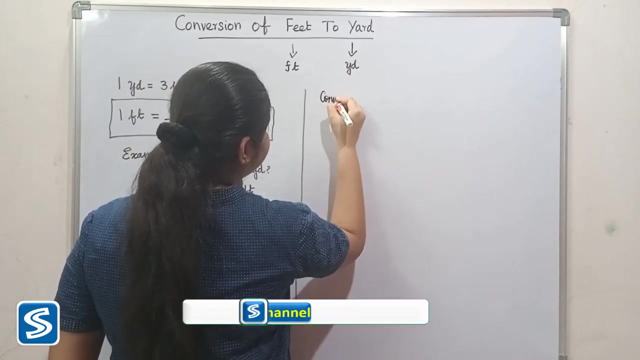 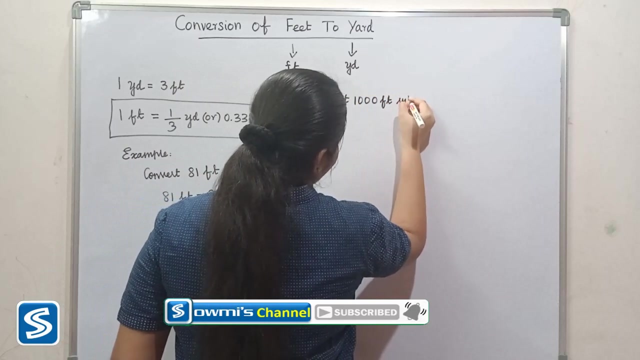 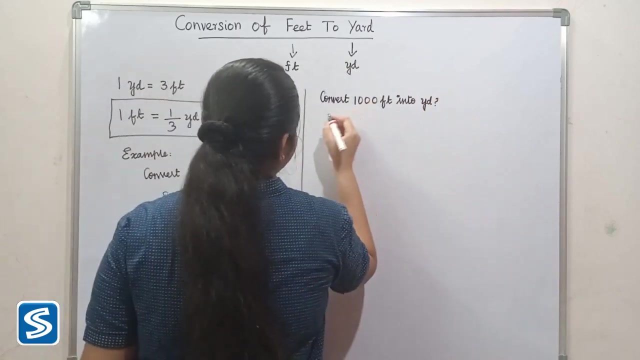 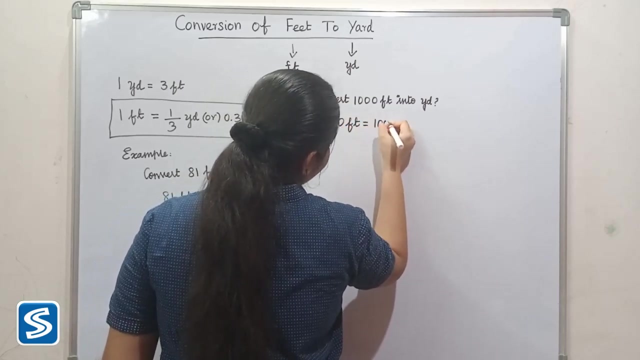 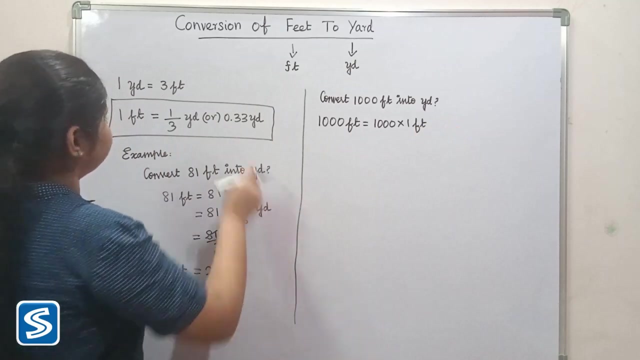 So 81 feet is equal to 27,. yeah, Next we will take another example. Convert 1000 feet into yard. 1000 feet can be written as 1000 multiply 1 feet. Now we have to substitute 0.33 yard in the place of 1 feet. 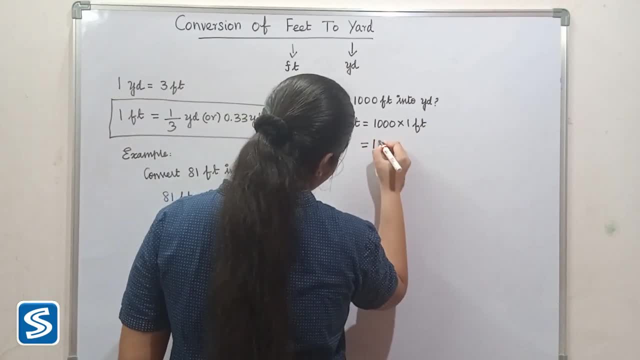 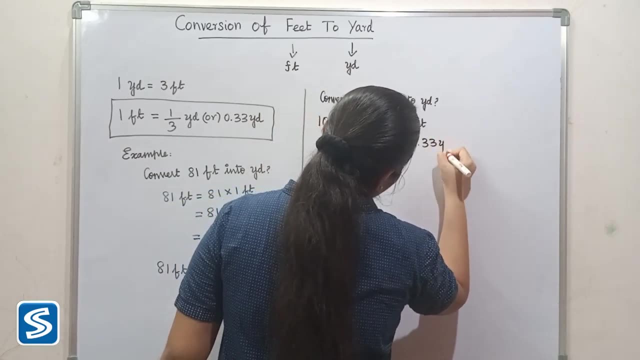 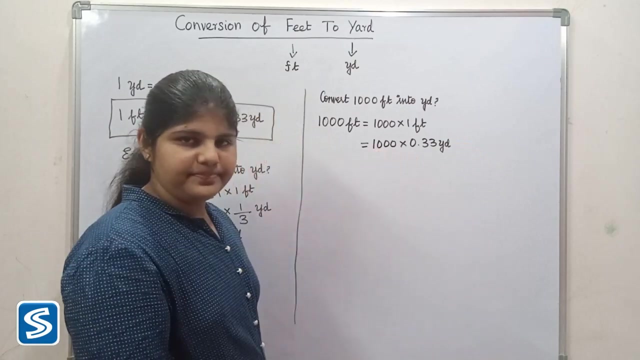 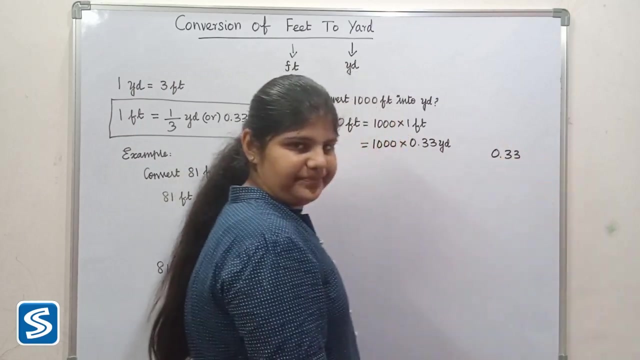 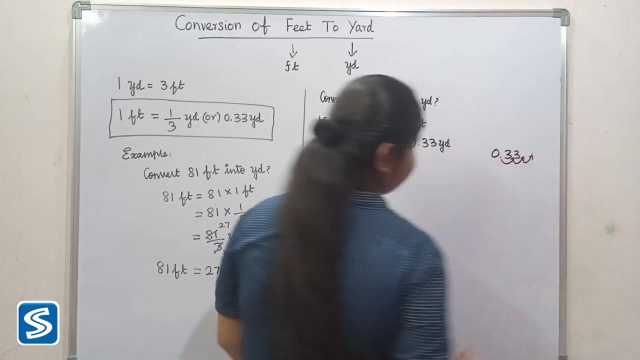 So 1000 multiply 0.33 yard. So the easy way to multiply by 1000 is to move the decimal point 3 places to the right, So 1,, 2, 3.. Now we have to fill 0's in the empty spaces. 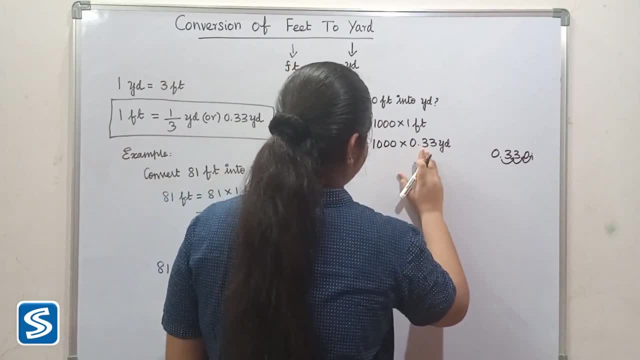 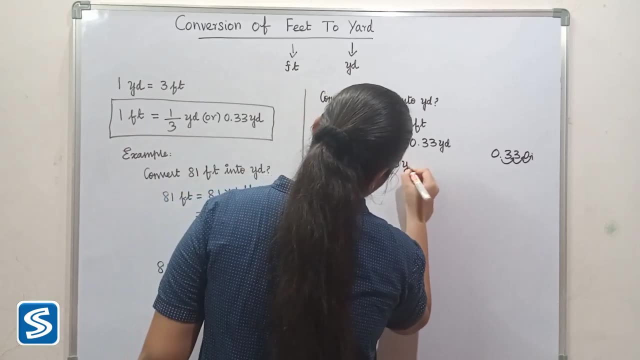 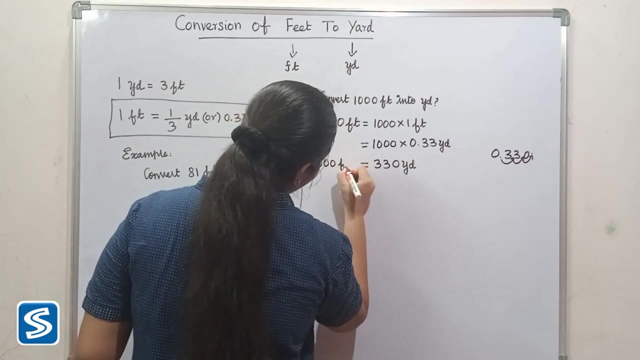 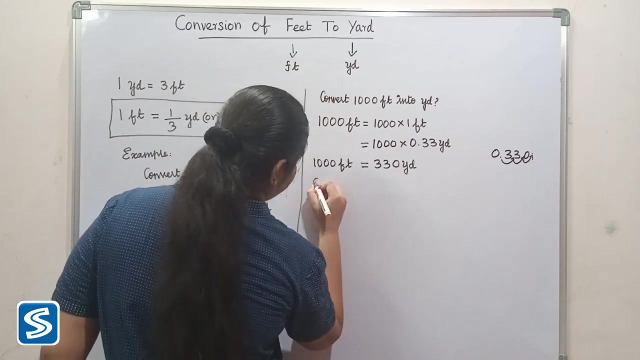 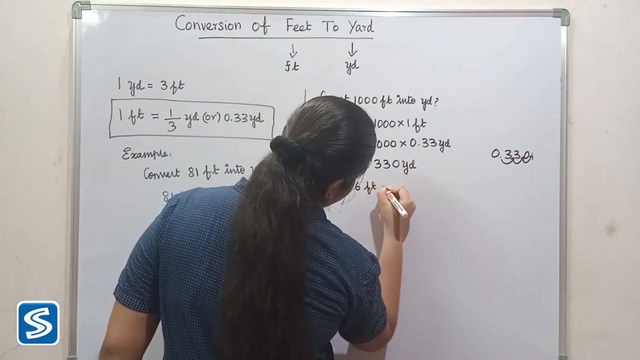 So when we multiply 1000 with 0.33 yard, our answer will be 330 yard. So 1000 feet is equal to 330 yard. Next we will take another example. Convert 56 feet into yard. 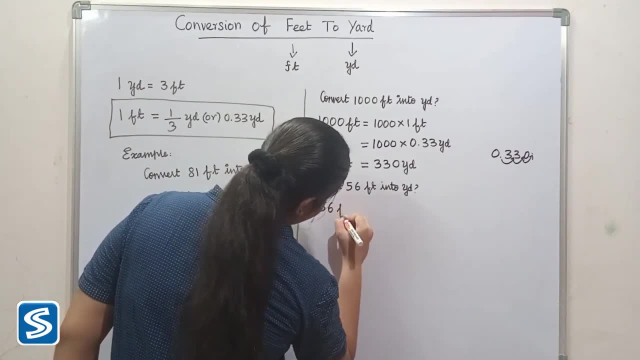 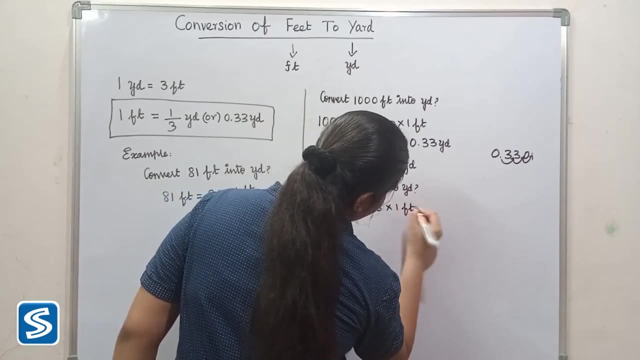 56 feet can be written as 56 multiply 1 feet. Now we have to substitute 1 by 3 yard in the place of 1.3.. So 1 by 3 yard harden into 56 by 1.3.. 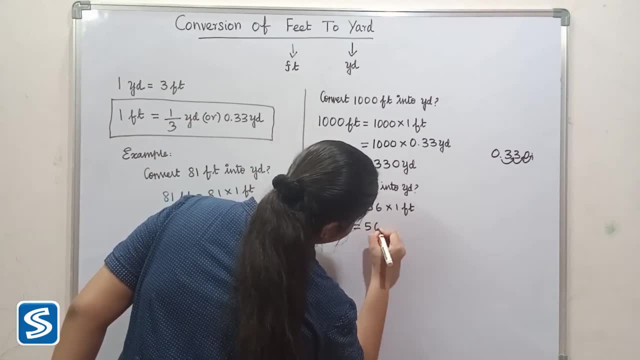 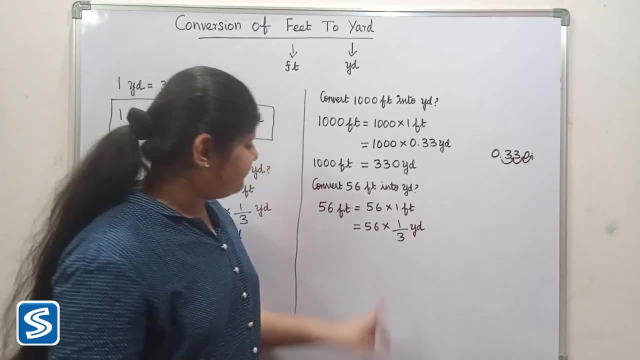 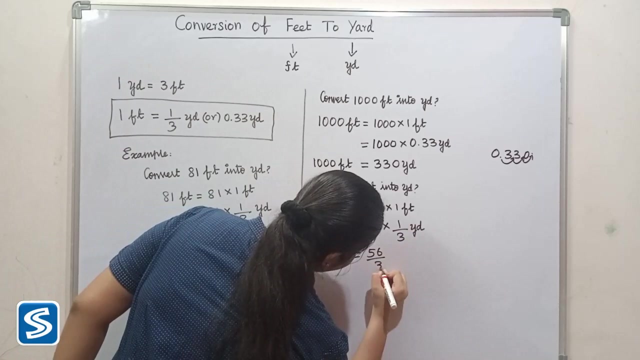 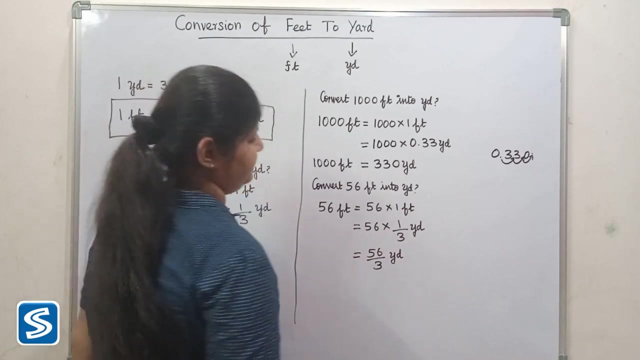 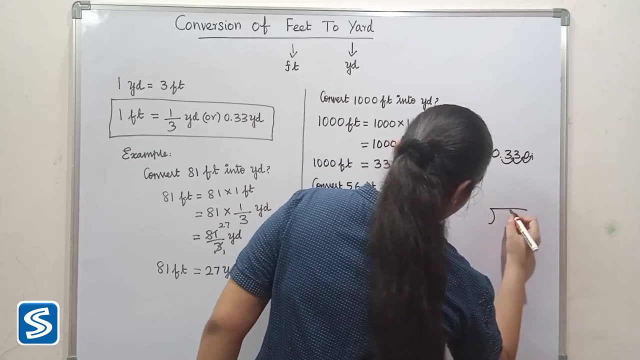 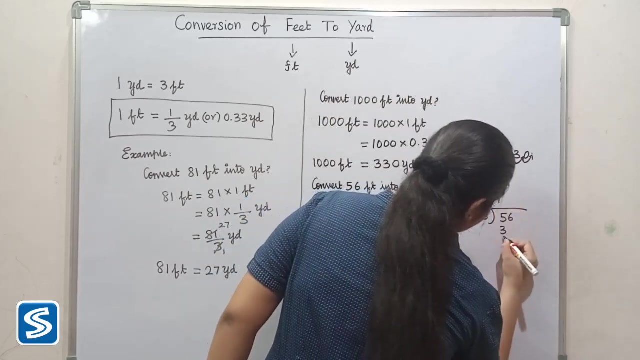 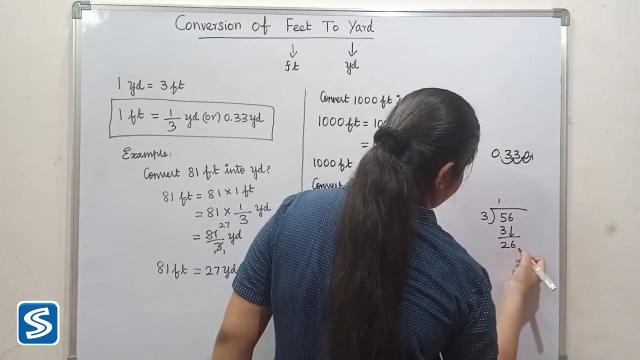 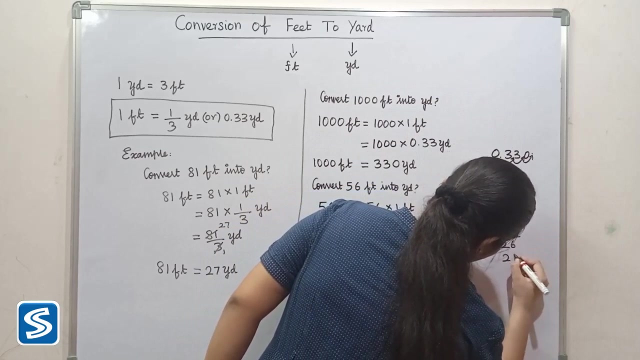 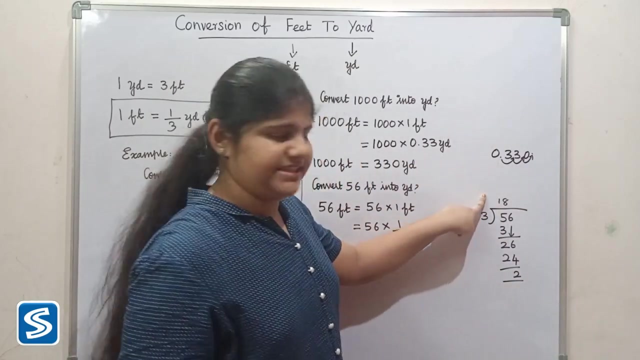 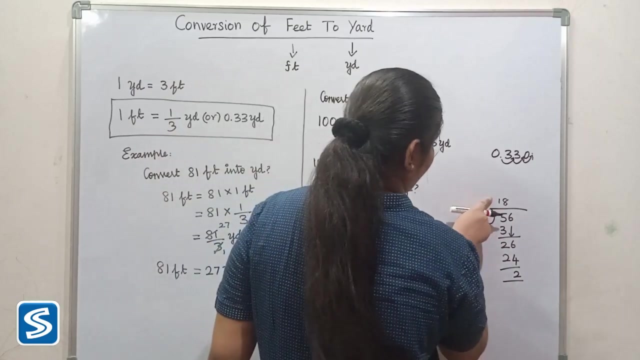 feet. so 56 x 1 by 3 yard. 56 x 1 will be 56, so 56 by 3 yard. now we have to divide 56 by 3. so now we have to consider quotient as yard and reminder as feet. so here the quotient is 18. so 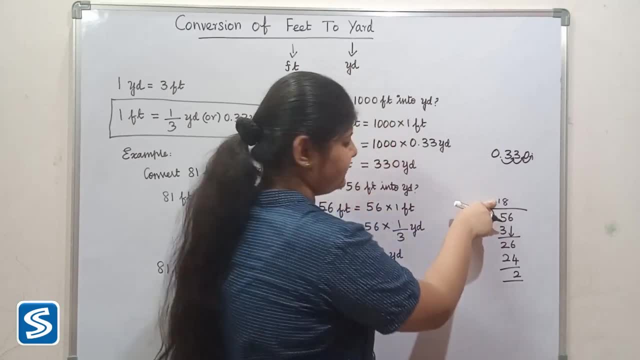 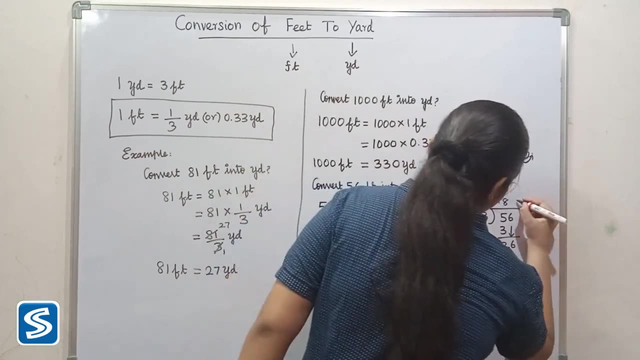 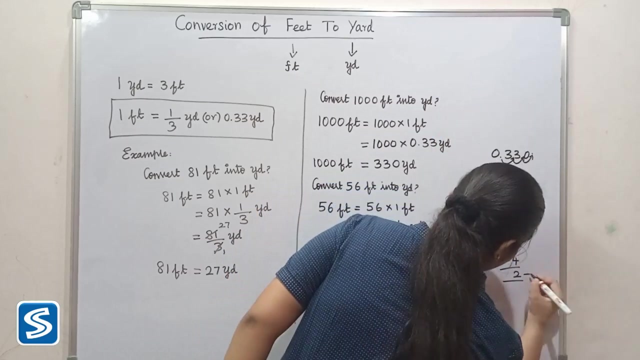 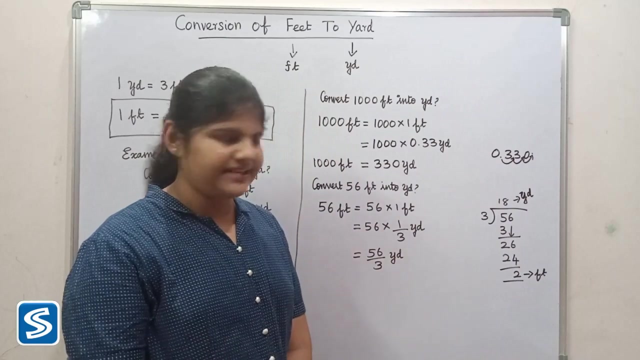 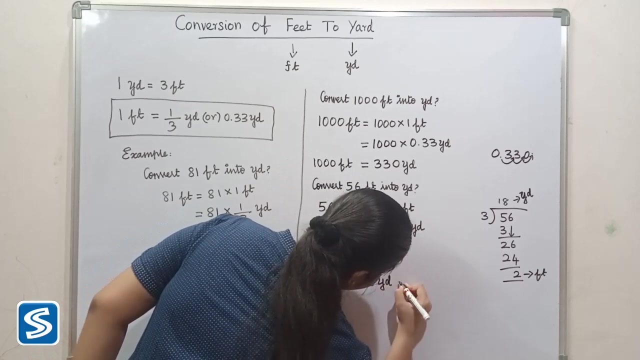 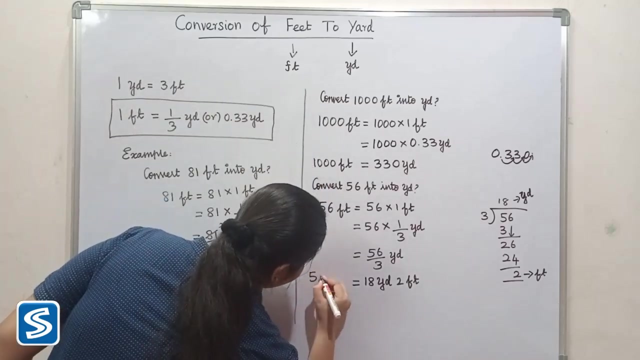 now we have to consider 18 as yard and here the reminder is 2, so now we have to consider 2 as feet. so when we divide 56 by 3 yard, our answer will be 18 yard 2 feet. so 56 feet is equal to. 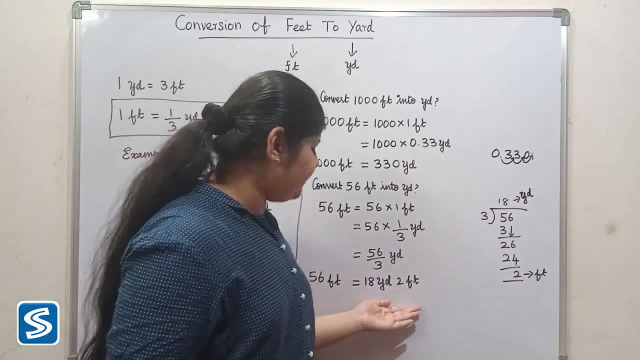 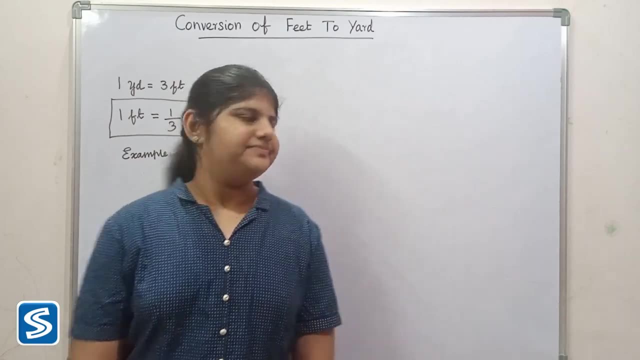 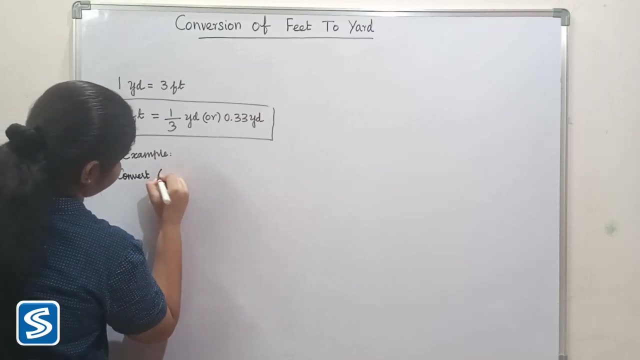 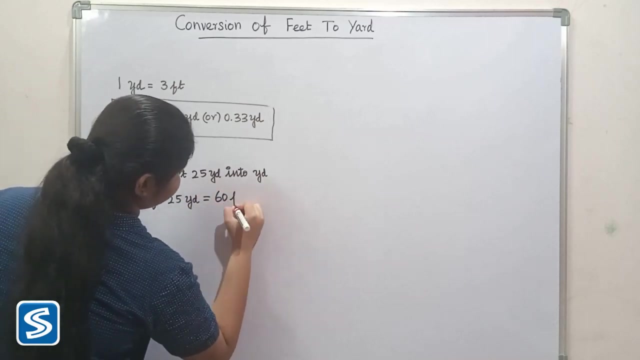 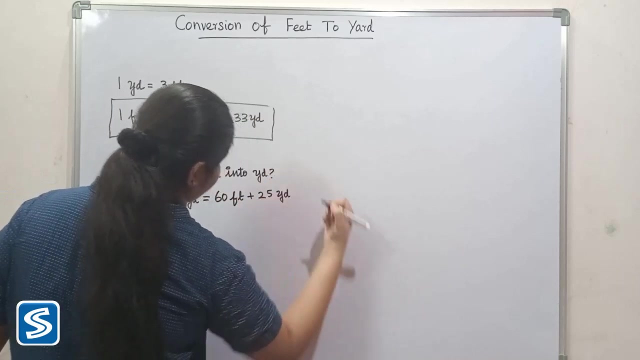 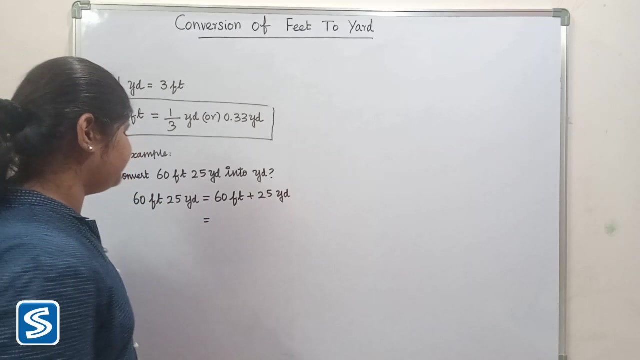 18 yard, 2 feet. next we will take one more example. for example, we can take convert 60 feet 25 yard into yard 60 feet. 25 yard will be 60 feet plus 25 yard. 60 feet can be written as 60 x 1 feet. 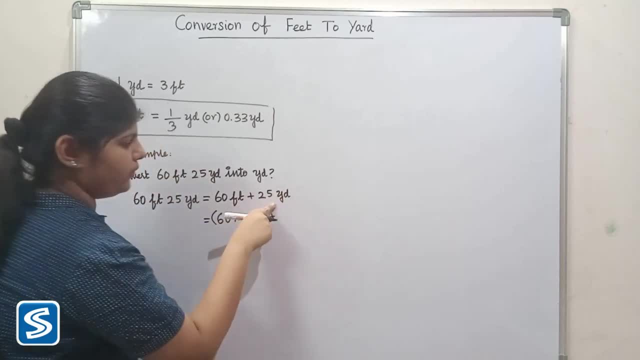 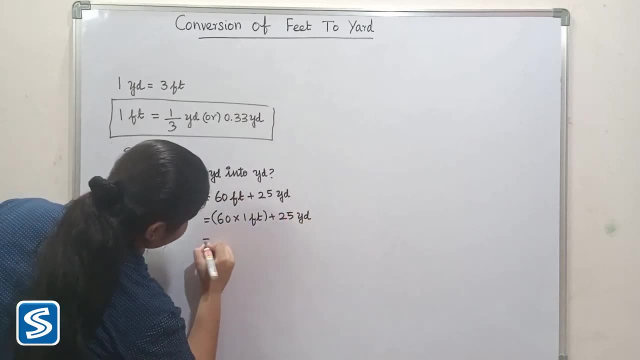 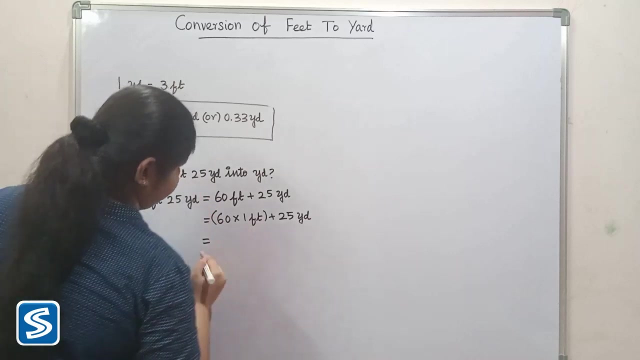 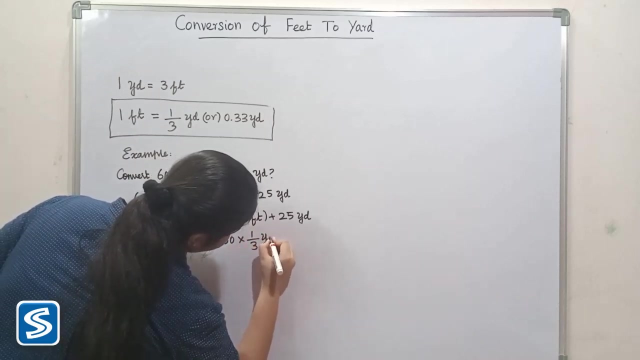 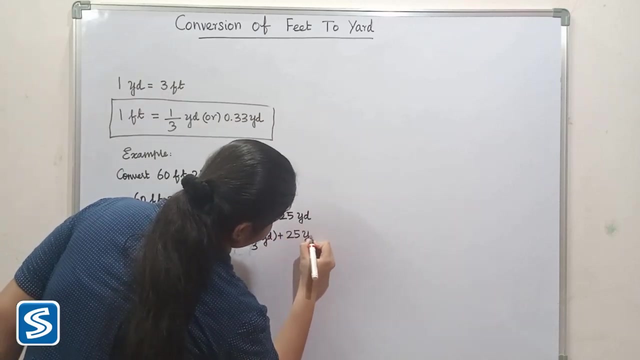 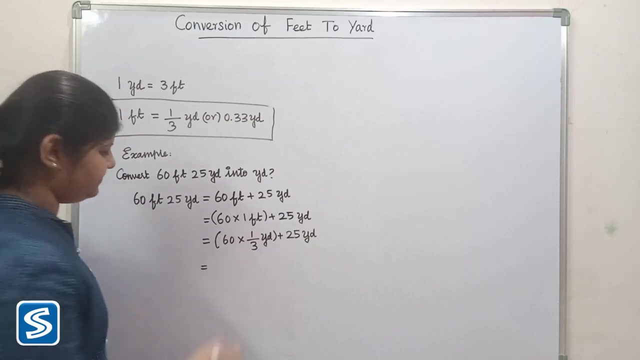 plus 25 yard. now we have to substitute 1 by 3 yard in the place of 1 feet, so 60 x 1 by 3 yard plus 25 yard. 60 x 1 will be 60, so 60 by 3 yard. 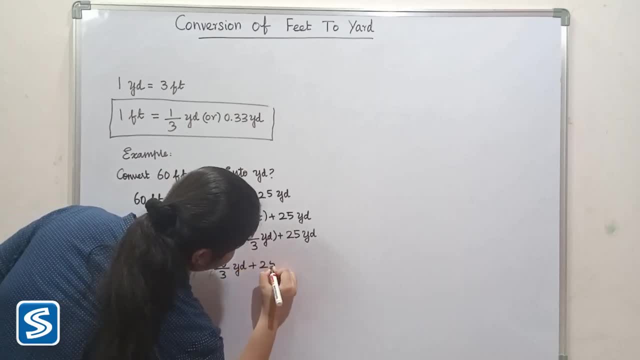 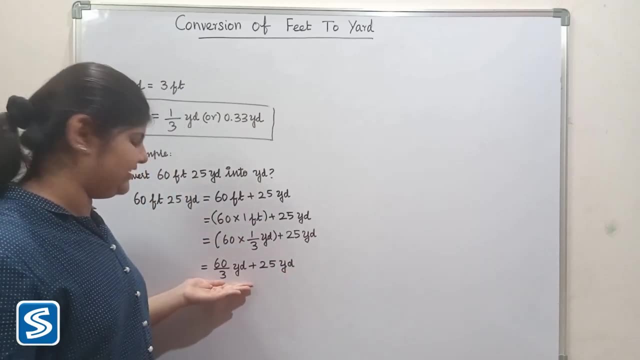 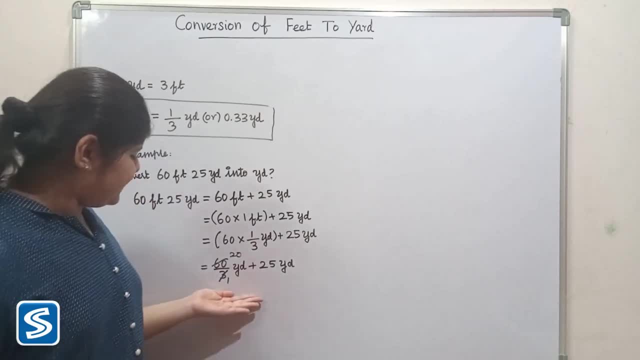 so 3: 1s are 3, 3, 20s are 60, so 3: 1s are 3, 3 2s. so 3: 1s are 3 by 3 yard and 2: 1s will be 5 yard. 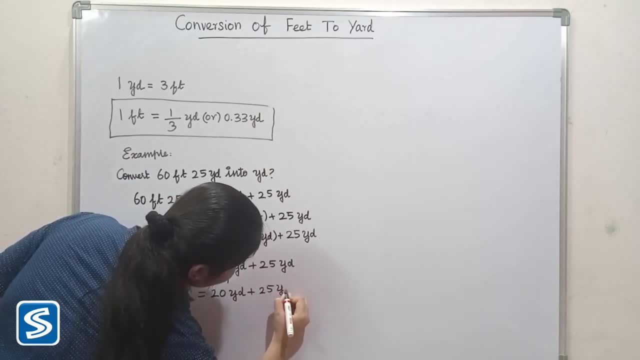 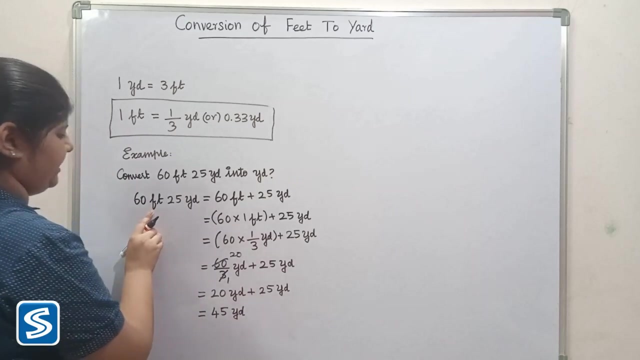 and 2: 1s will be 4 yard and then 8 yard will be 6 yard. so 3: 1s can be written as 5 yard. so 10 x 10, so 6 inch dome is 6立 благ.